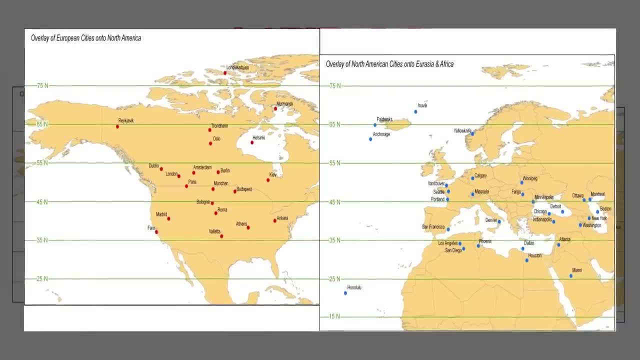 interesting to see how the latitude of the continent is compared to the latitude of the United States. It's very interesting to see the overlay of the European cities on top of the US territory and vice versa, For instance, as stupid as it may sound, I had no idea Reykjavik was as 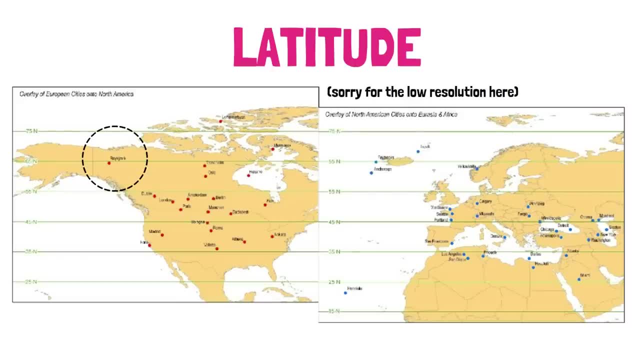 further north as Northern Canada. The same applies to Oslo. It makes sense that Portuguese and Spanish cities are on the same level as California, at least climate-wise, But it's weird, for instance, that Ankara is at the same level as Delaware, For some reason. I always thought it was so much. 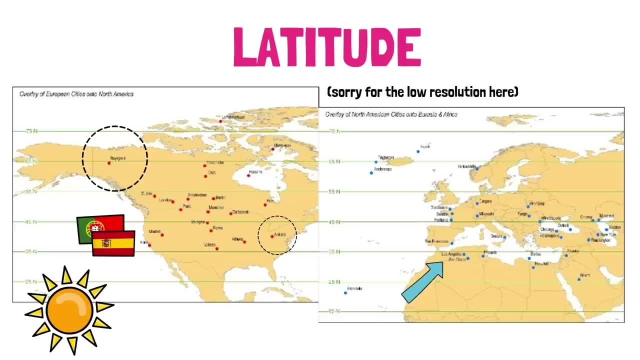 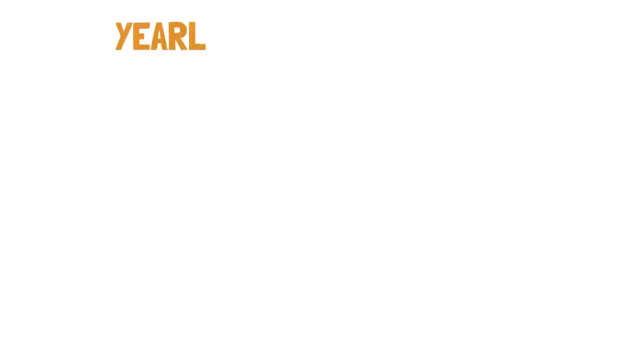 further south. It's also strange to see that Los Angeles is on the same latitude as the United States As Algeria and North Africa, But that New York is at the same latitude as Azerbaijan. Speaking of Portugal, Spain and California, how do the US and Europe compare when it comes to the? 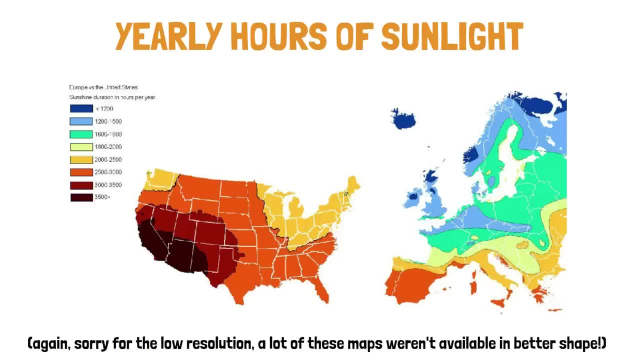 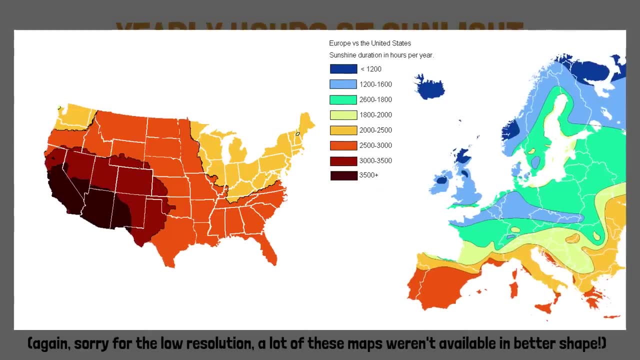 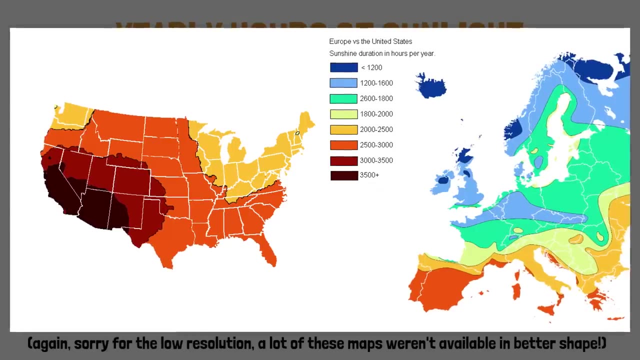 hours of sunlight they get every year. Through this map, we understand that the Southwest USA gets more hours of sun than anywhere in Europe- over 3,500 a year- And, unlike Europe, there's nowhere in the US that gets less than 1,800 hours of sun, as is the case in many areas of Europe. 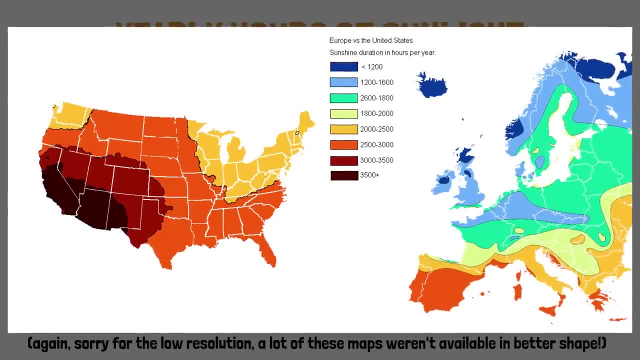 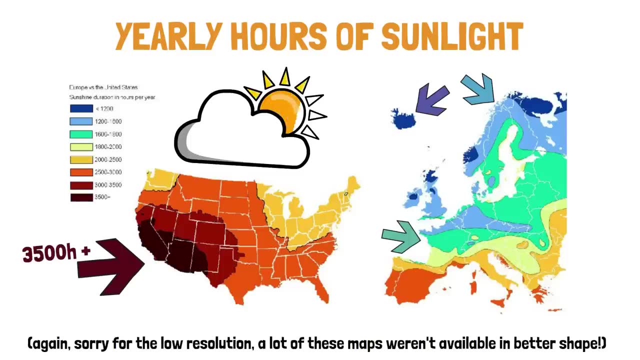 those in light, green, blue and dark blue. It's also odd- at least to me, who isn't an expert on this matter- how the amount of hours of sun isn't directly related to the latitude of the region. I always assumed that the closer to the 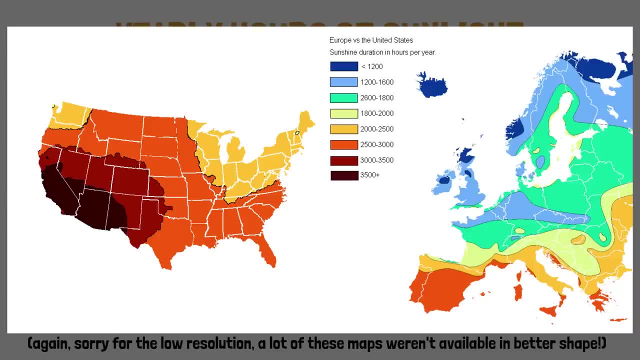 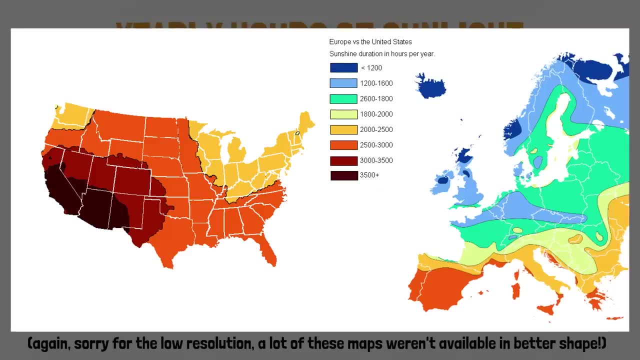 equator you are, the more hours of sun you get. But we can see on this map that this isn't the case at all, Even though we can tell that usually southern areas get more sun. If you know which other factors determine hours of sun, let me know in the comments. Another interesting topic is: 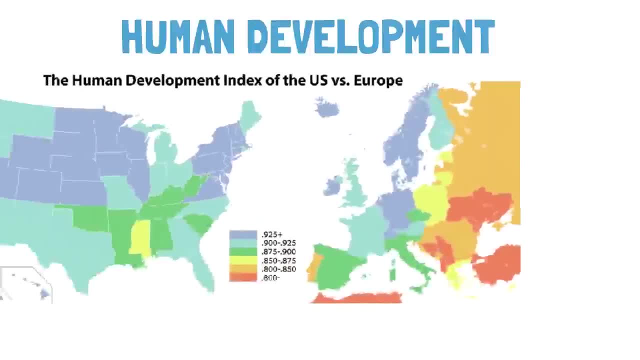 human development. The United States and Europe are arguably two of the most developed areas of the world. The United States and Europe are arguably two of the most developed areas of the world. The United States and Europe are arguably two of the most developed areas of the world. This. 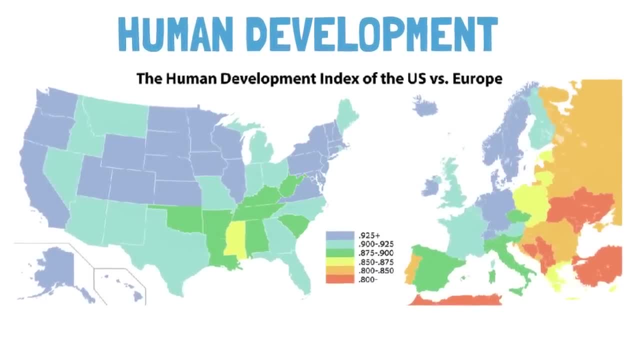 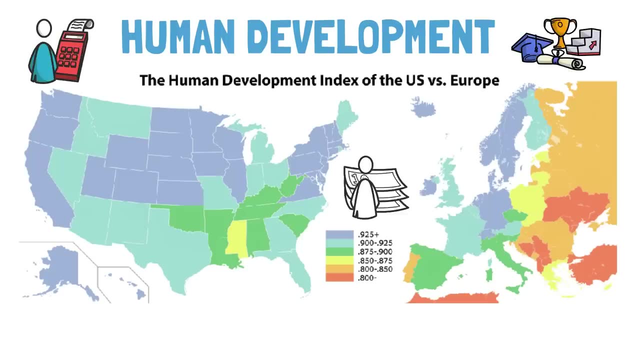 map compares the human development index of each US state and each European country. In case you don't know, the HDI is calculated as the geometric mean of life expectancy, education and gross national income per capita, Assuming that those indicators are representative of the quality of 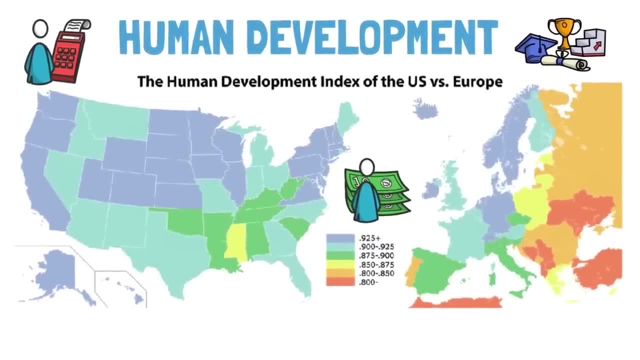 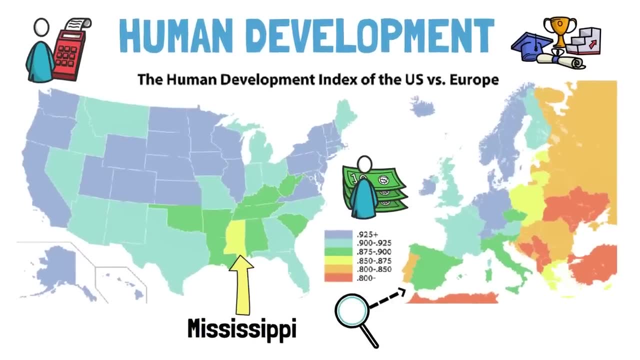 life of people. it seeks to measure precisely that. In the United States, there's only one state that doesn't make it into the top three HDI categories: Mississippi. When we look at Europe, only a handful of countries are in the top ranking: Iceland, Norway and the United States. 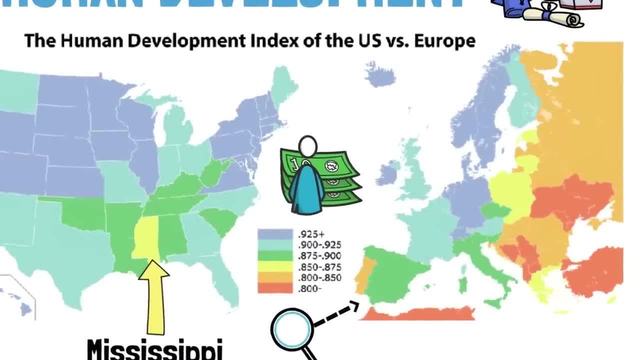 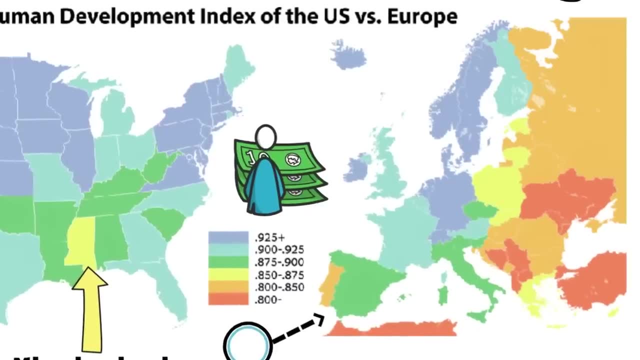 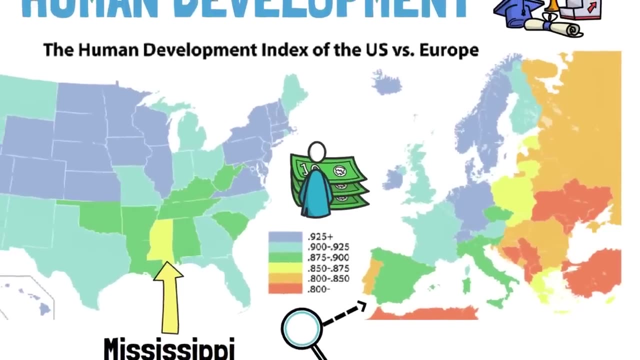 Sweden, Ireland, Denmark, Germany, Netherlands and Switzerland. And when you look at Eastern Europe, these levels go significantly down, with many countries in the lowest category, such as Ukraine, Turkey, Serbia, Bosnia-Herzegovina, Albania and North Macedonia In Western Europe. 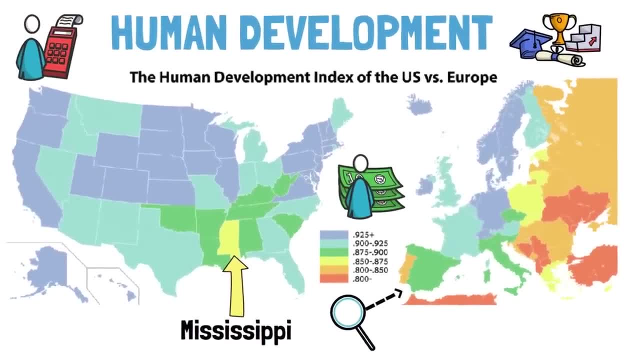 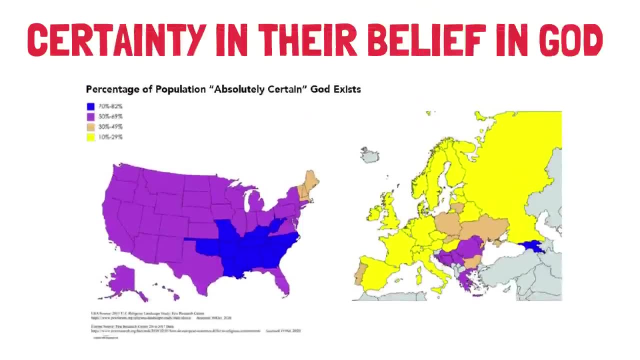 Portugal is the only country who isn't in the top three levels of HDI. A somewhat subjective comparison of these two areas is also depicted in this other map. This is based in a 2014 Pew Research Center poll. It's almost 10 years old, so the data might be somewhat outdated and 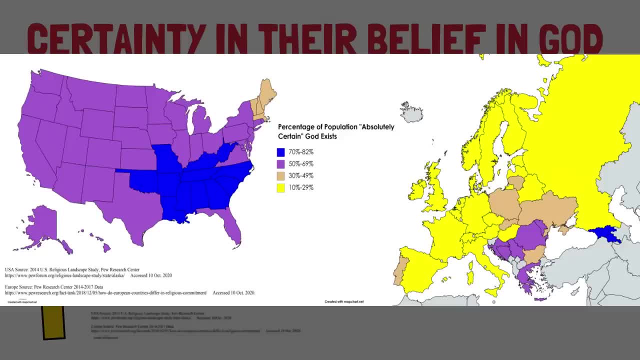 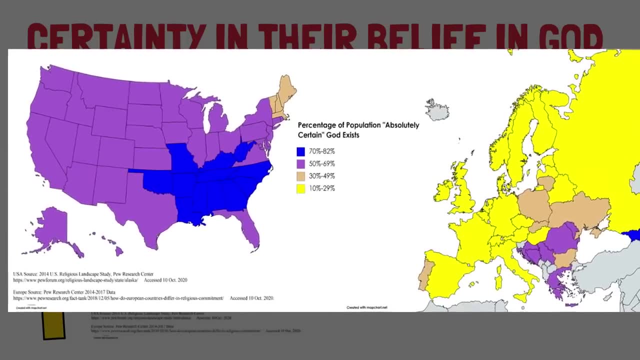 no longer valid. Always keep that in mind for these types of videos where data and maps are presented. The data might not be 100% right and it might be outdated, But in this one, people were asked if they are absolutely certain of God's existence, And the comparison of the results. 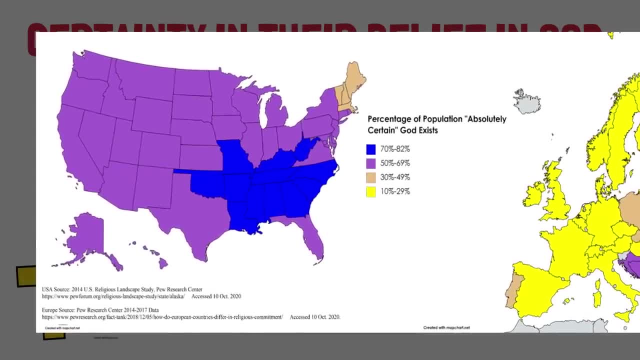 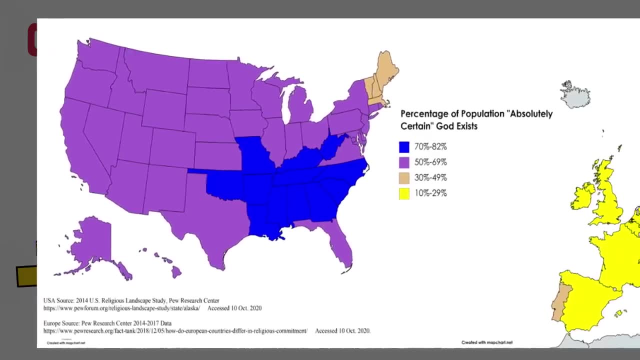 between the US and Europe is astonishing. The majority of US states have over 50% of people being certain of God's existence, some even surpassing 70%. Those in dark blue- Only Vermont, Maine and Massachusetts- have results under 50%. 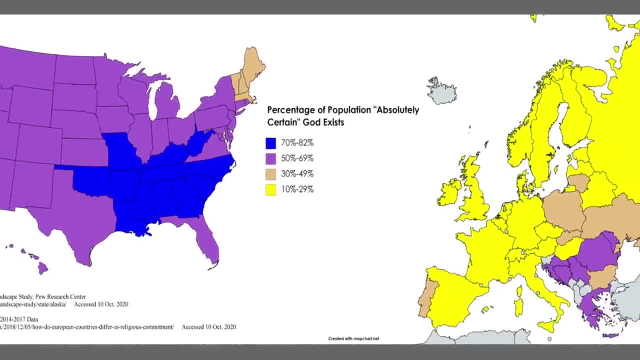 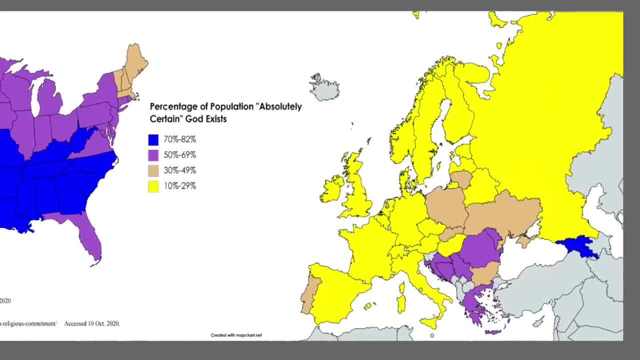 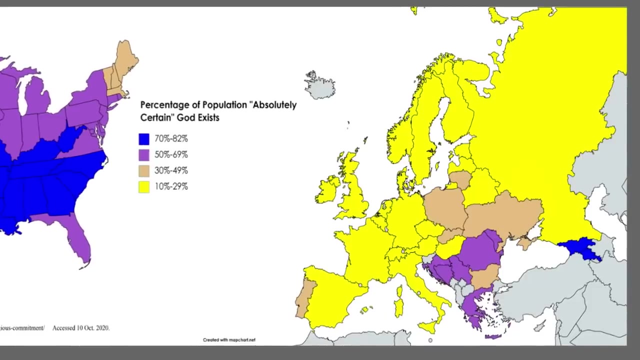 while most of Europe is much less certain in their belief of God, Most of the continent is in yellow, with only 10-29% being certain of their belief. Portugal, Poland, Slovakia, Lithuania and Ukraine, along with Bulgaria, go up to 30-49%, but still not reaching over half of the population. The 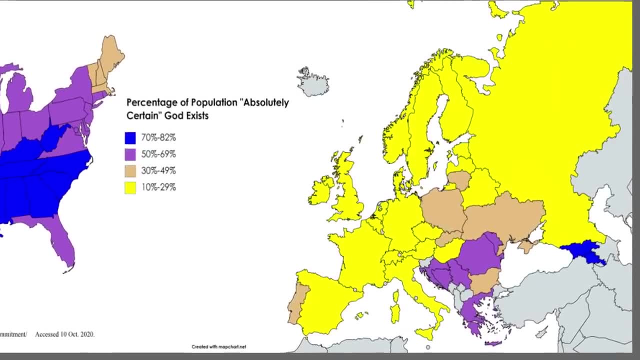 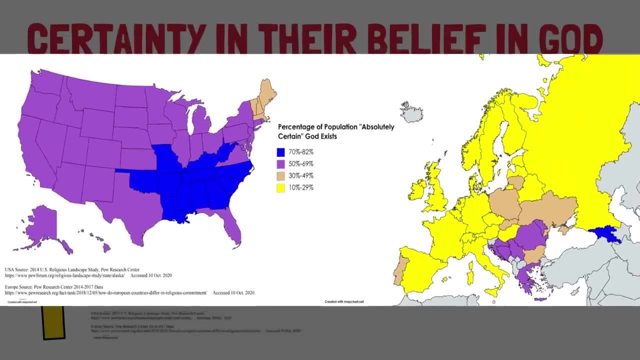 rest of the Balkans is more religious, but it's only Georgia and Armenia who reach the dark blue level. There's a few countries missing from the top three, but it's not a big deal. This map those in grey. if you have any idea of how religious they are, leave a comment below. 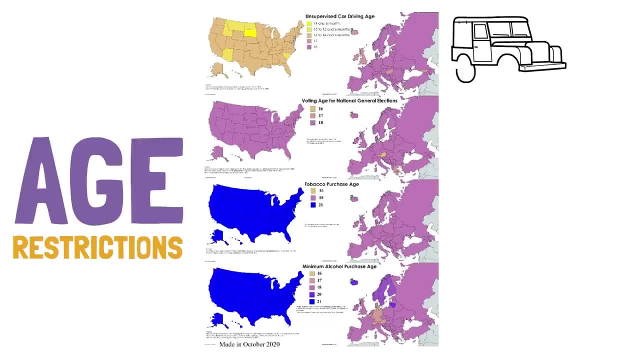 Another interesting thing we can compare are age restrictions. in the US and Europe, Age restrictions can be applied to driving, voting, tobacco or alcohol purchases. Many of these change often, so be aware these might not be correct at the moment you watch. When it comes to 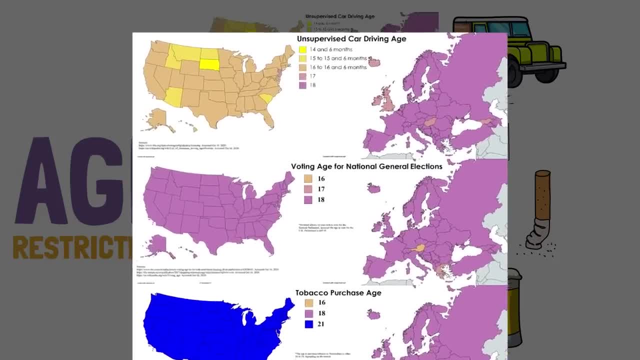 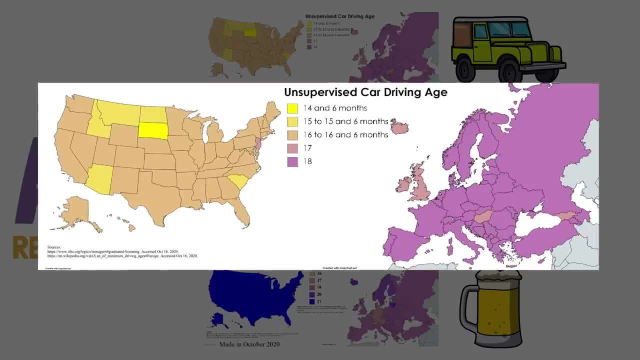 driving. the US government allows people to drive at a much younger age. In South Dakota it says you can drive at 14 years and 6 months. That's kind of crazy. if it's true, The oldest driving age seems to be New Jersey at 17.. While in Europe the vast vast majority of countries has an 18. 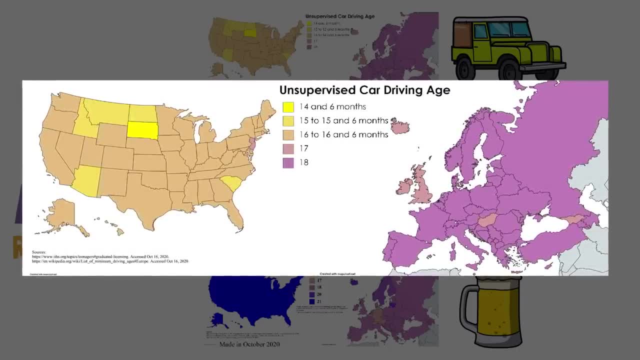 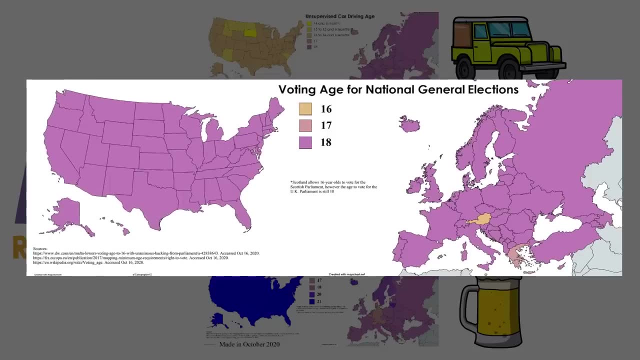 years minimum driving age. Only the UK, Iceland, Hungary and Georgia have lowered it to 17.. When it comes to voting, 18 is common all around. Only in Europe are there two countries that differ: Austria at 16 and Greece at 17,, although I'm not sure if these limits are the same for all types. 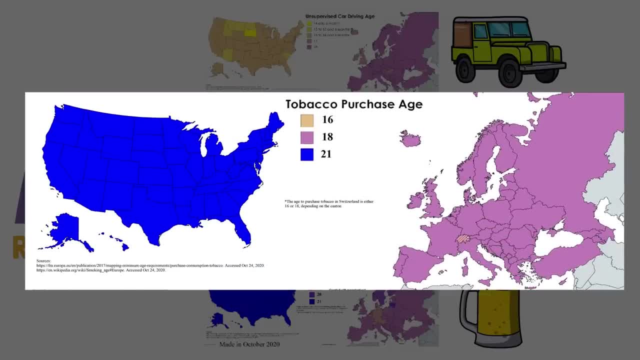 of elections. Tobacco purchase is technically only allowed over 21 in all of the US, while in Europe you can buy it at 18.. Alcohol purchase is only allowed over 21 in all of the US, while in Europe you can buy it at 19.. Alcohol purchasing is also forbidden for people under 21 all across the. 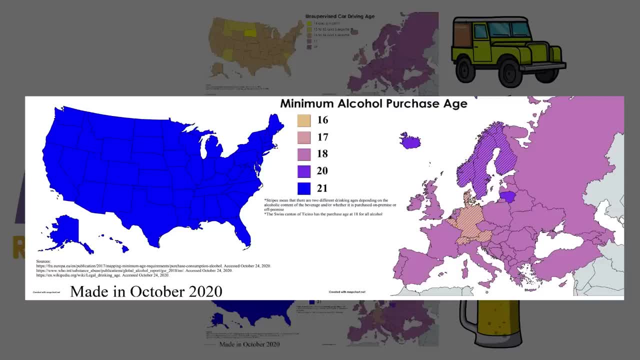 United States, with the limit ages varying a lot across Europe, but none being higher than 18 or 20, although, again, this also varies depending on the type of alcohol. For instance, in Portugal, I think, you can buy beer or wine as long as you're over 18,. 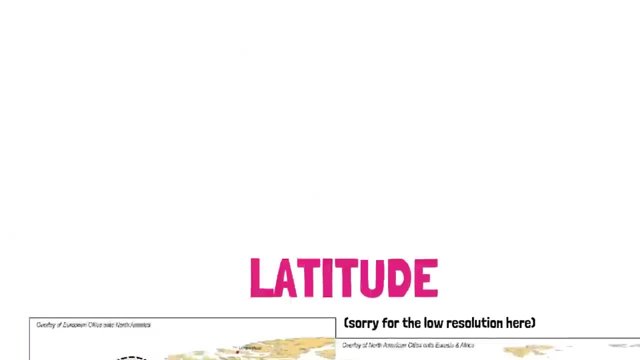 but other drinks do have a 20 year age limit. I think When it comes to comparison between military, for instance, it's a difficult comparison to make. Ecom Empire has Megalovania, Mesopotamia and Cahoumera. According to Wikipedia, 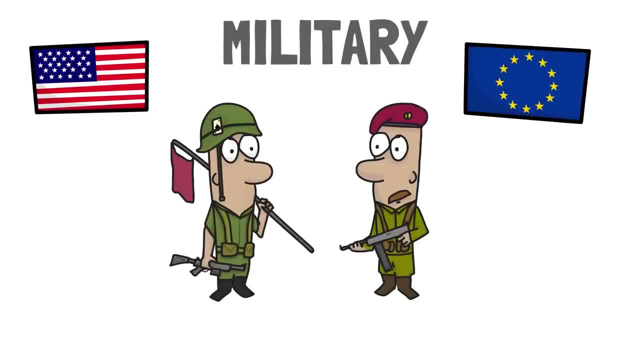 the US army has a personnel of around 1 million, counting active troops, reserves and National Guard. Ahh, he's refering toFoxia. fairly quote, unless maybe you're interested in, and according to this 2018 article from Business Insider, the top five strongest militaries in. 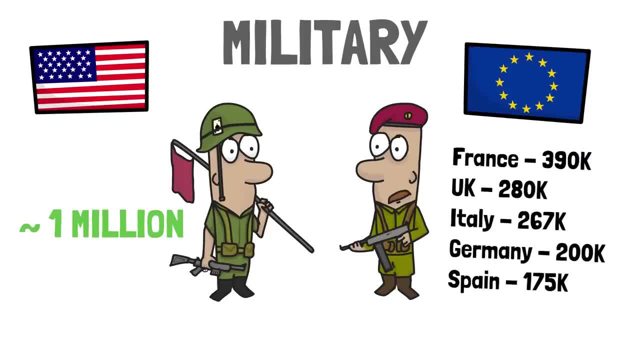 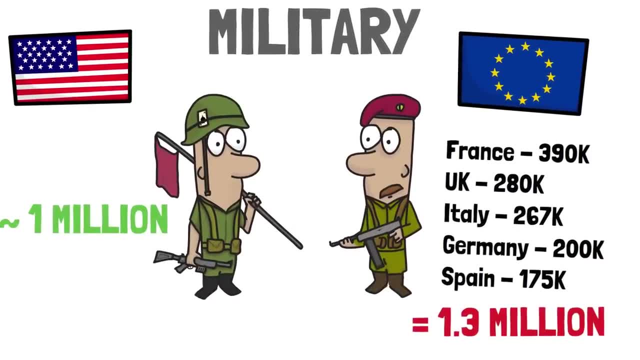 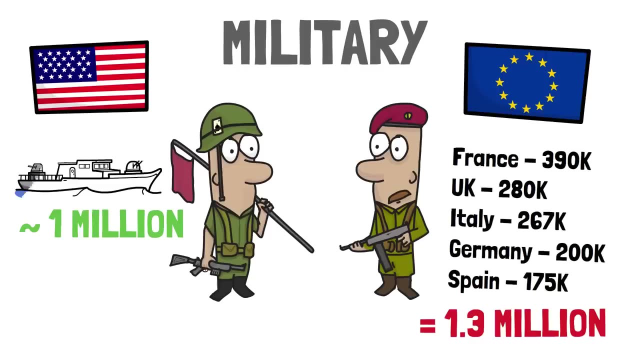 Europe- all of these maps exclude Russia- are France, with 390,000, the UK 280,, Italy 267,, Germany 200, and Spain 175.. Together, these alone would surpass the US Army, although you'd still need to take into account the material advantage of the US Ships, intelligence tanks, planes. 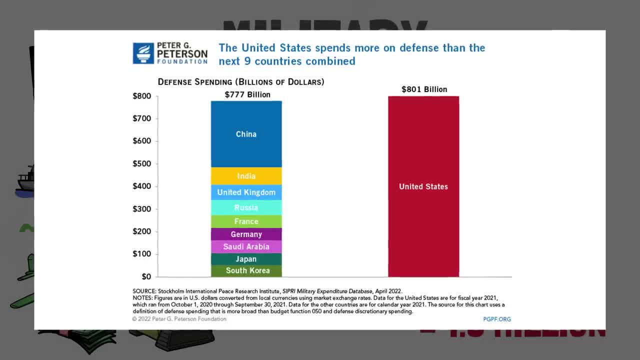 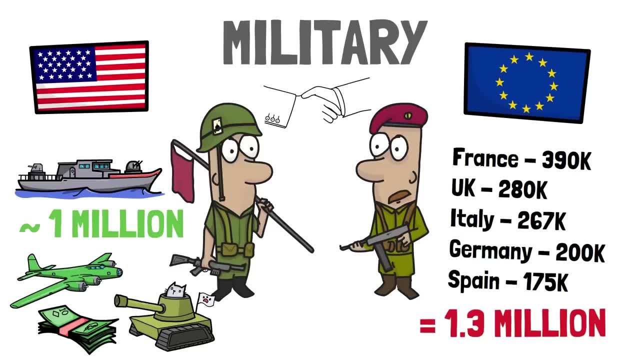 investment, and in these the US has a considerable advantage, as we can see from this graph depicting the investment comparisons. But thankfully most of Europe and the US are allied through NATO, so a comparison isn't needed because in the event of a conflict, 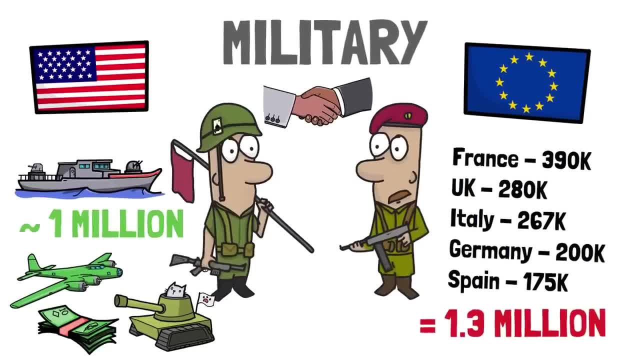 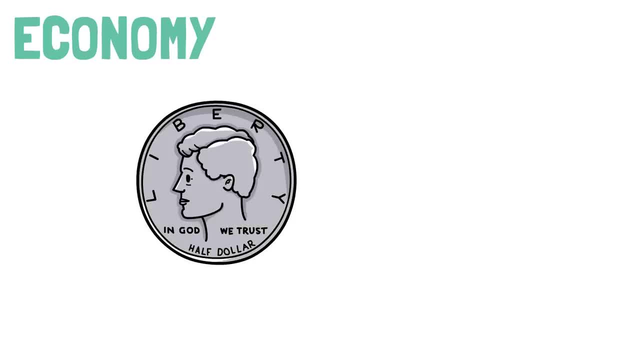 it is very likely they would be on the same side. And what about an economic comparison? The United States and the European Union are the two largest economies globally in nominal terms In recent years. only in 2011 did the European Union have a higher GDP than the US. keep in mind. this exclusively, And in the past the US has had a higher GDP than the US, but in the past, the US has had a higher GDP than the US And in the past, the US has had a higher GDP than the US. 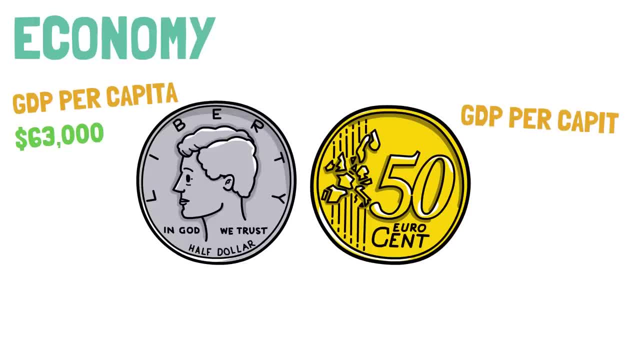 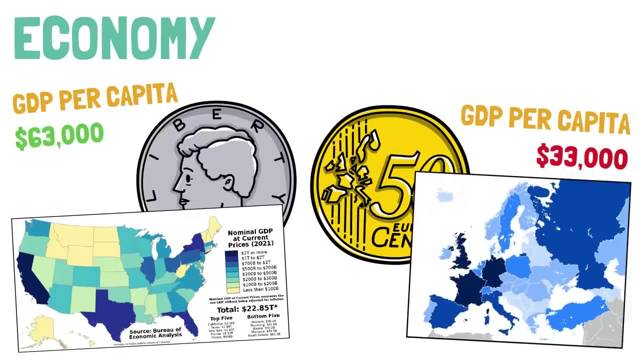 non-EU Europe. The US's GDP per capita is 63,000,, while in the EU it's 33.. But keep in mind, both of these are on average. there are EU countries and US states with higher and lower values. Also, as we can see from these maps, the US's GDP is mostly carried by California. 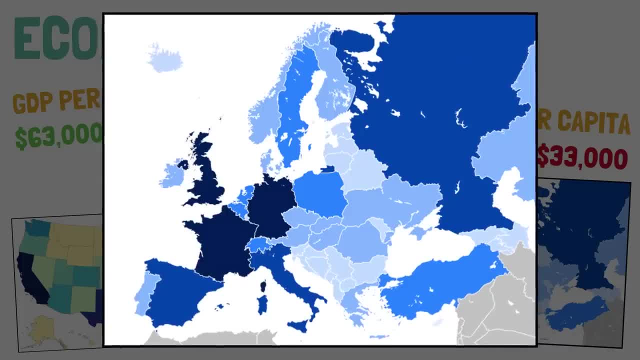 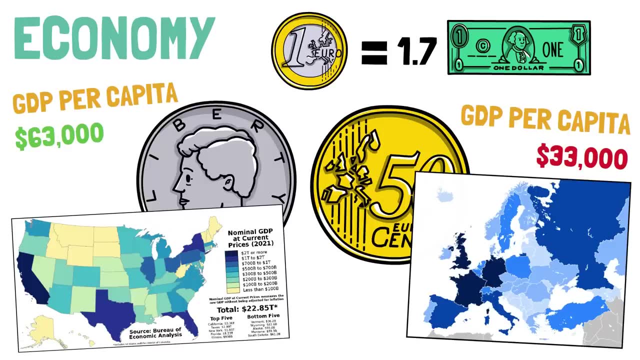 Texas, Florida and New York, while Europe's is mostly carried by France, Germany, the UK, Spain and Italy. When it comes to currency comparison, as I make this video, 1 euro equals $1.07.. The euro is mostly carried by France, Germany, the UK, Spain and Italy. 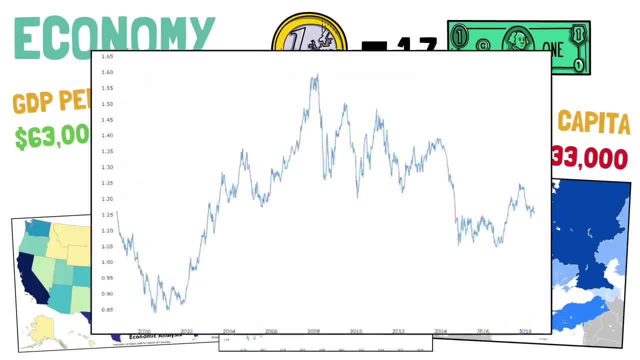 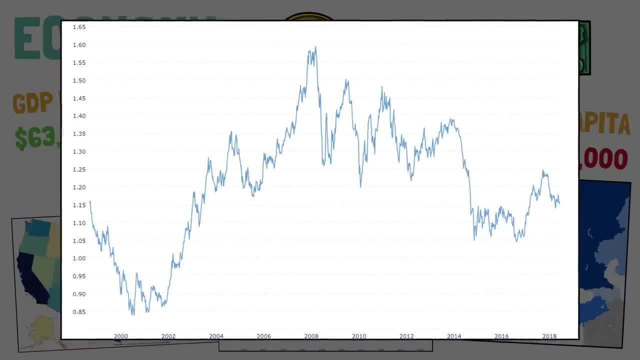 The euro's value has been higher and recently its value has decreased a little, approaching parity with the dollar, As we can see from this graph. there was only a short period in the early 2000s when the euro was worth less than the dollar, And there was a point where it was. 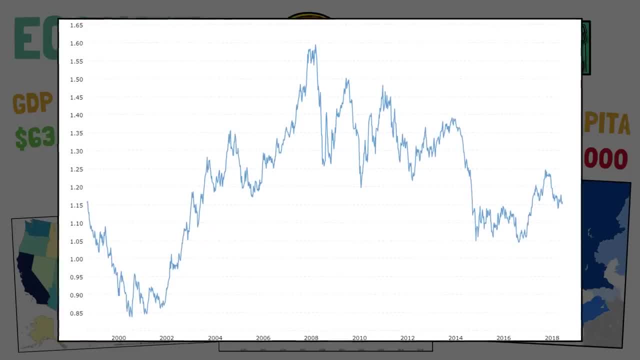 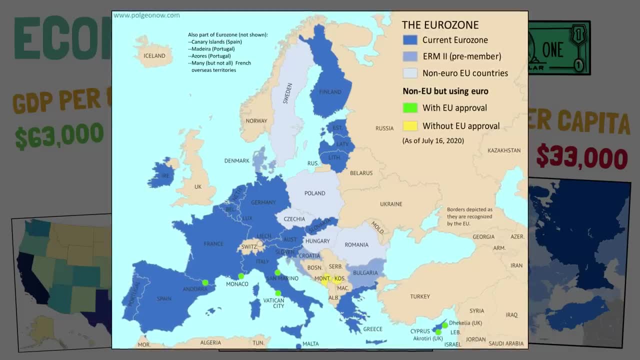 almost worth 50%. more Recently, things have stabilized and they're almost worth the same, But with Croatia joining the European currency next year, it might go up again. Also, keep in mind: not all of Europe, and not even all of the EU, use the euro as their currency. 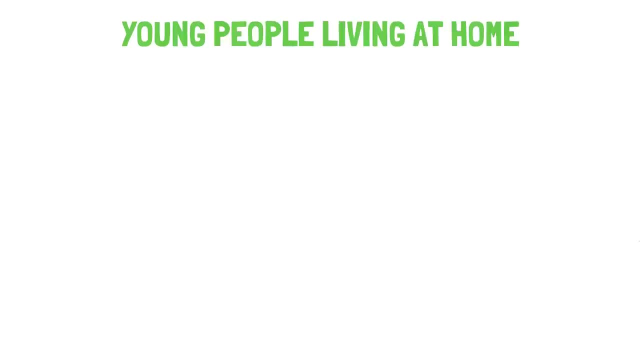 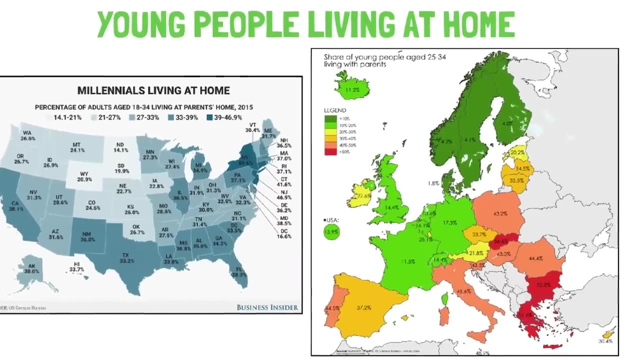 Another interesting point to compare is the percentage of young people aged 18 to 34 that still live in their family's home, Meaning. in most cases, they do not yet have the financial stability to live on their own. Both of these maps have data from 2015,, but from 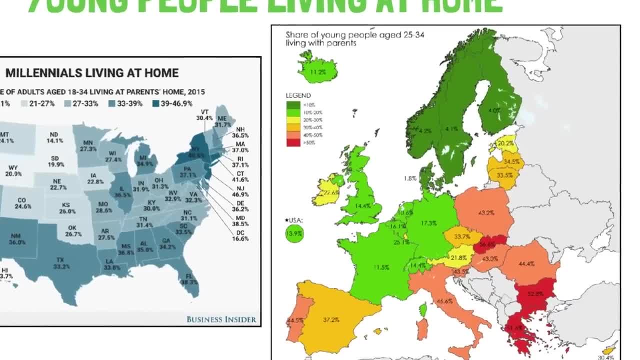 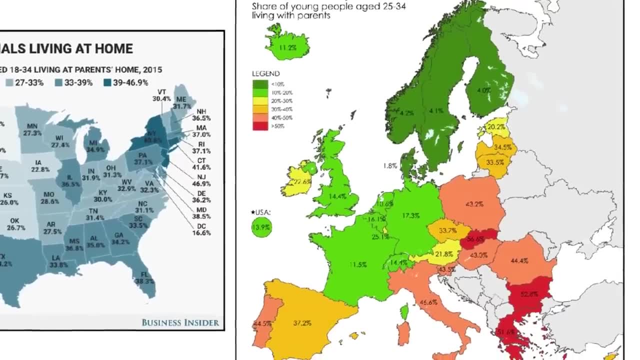 the most recent information I could find about this, the numbers haven't changed a lot In Europe. Nordic countries have very low values. They're also the highest income areas, so it makes sense people can more easily afford to live on their own. But it might also have to do with the cultural 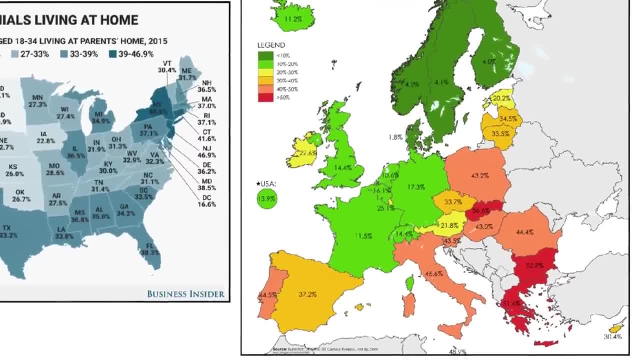 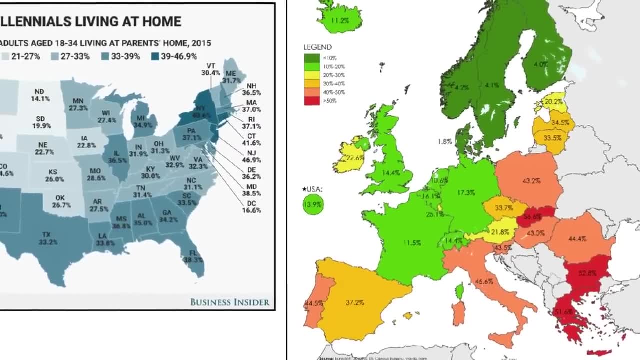 element In Southern Europe. the amount of young people still living at home is tremendous: 44% in Portugal, 37% in Spain and 46% in Italy, For instance, while Greece, Bulgaria and Slovakia are all above 50%. In the US, values are equally. 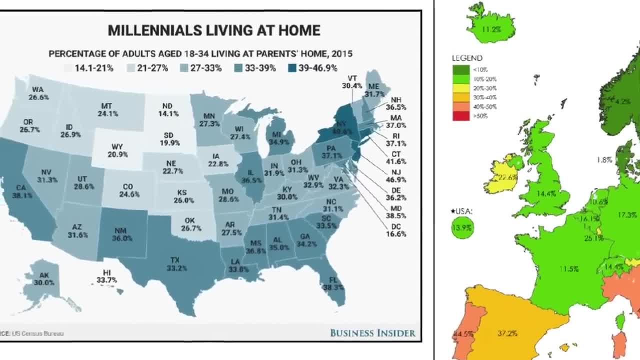 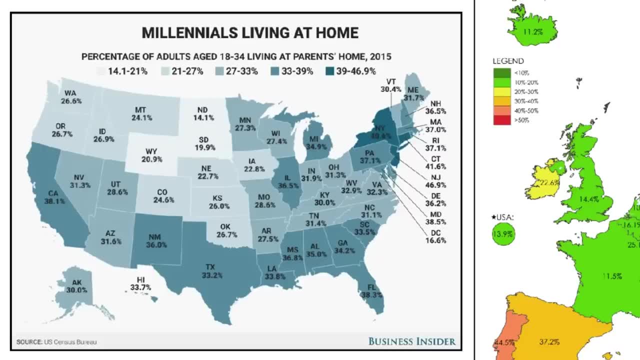 as high, with the difference being that there are no states at all below 10%. The lowest value is 14% in North Dakota and the highest being in New Jersey with 46%, although non-surpassed 50%. These high values are usually connected with the fact that salaries do not pay enough. 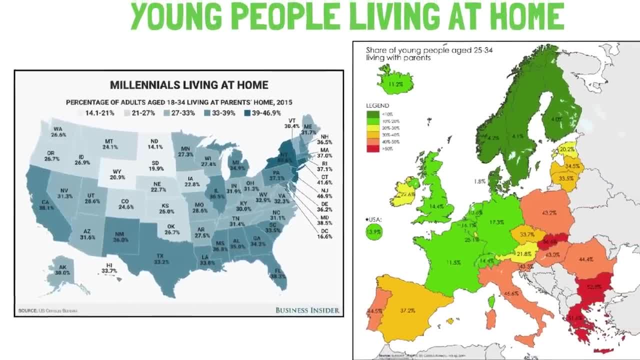 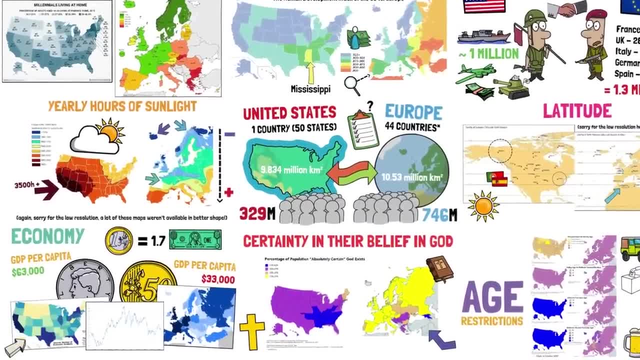